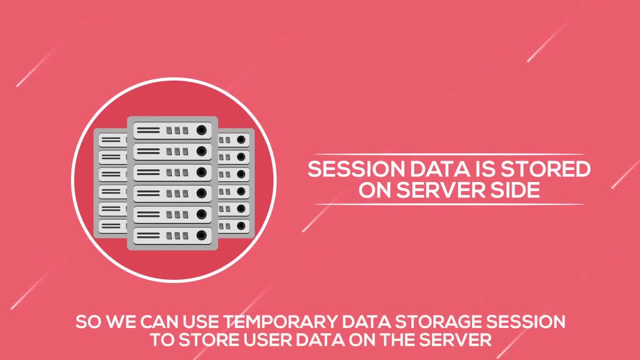 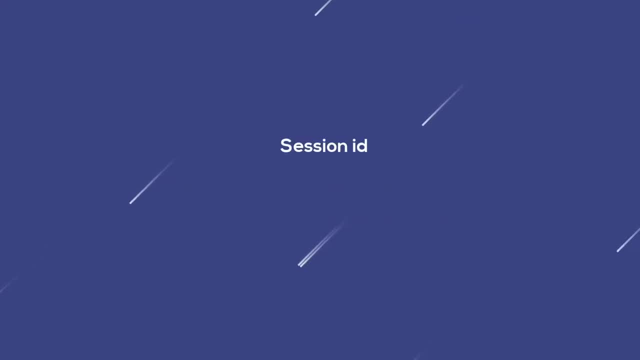 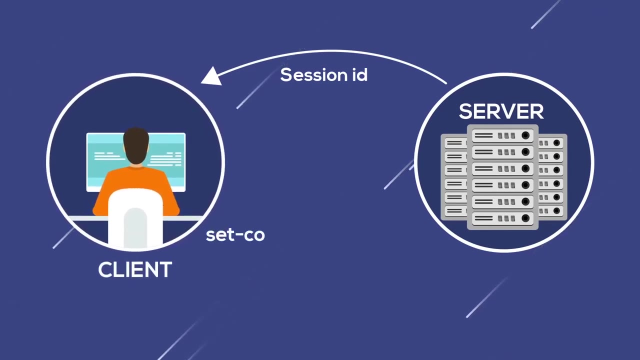 the session to store user data on the server. So how's that happen? Well, sessions, like I said, are generated on the server And the session ID gets sent back to the client in the cookie. So that cookie is set in the HTTP header and it gets sent back to the client in the cookie. 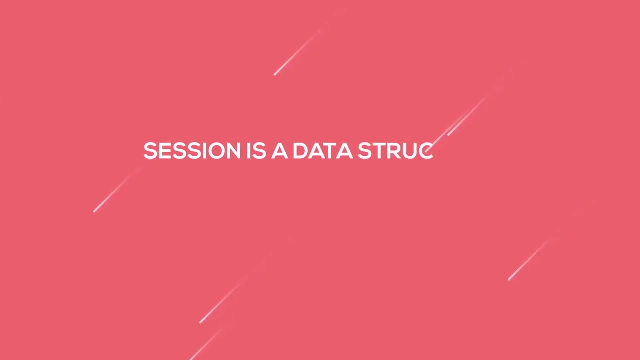 So the session is a data structure that stores user information. It's temporary data. I want you to remember this. Sessions are short lived And it is specific To one user only. So if you're on multiple devices, you and you log into in each device. 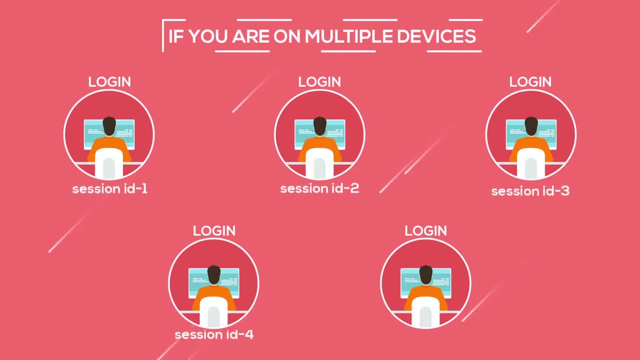 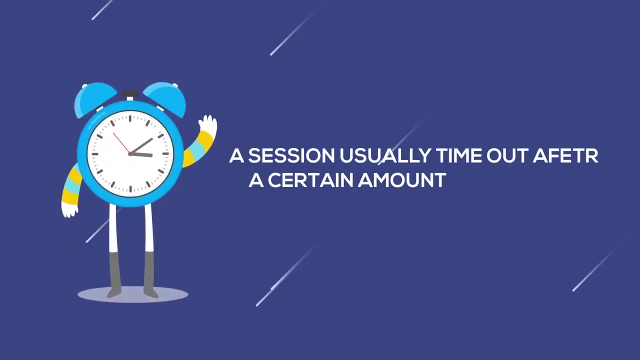 to the same application. you'll have multiple session IDs for each device Session IDs. like I said, they're managed on the server and then they pass to the client. they pass back to the client. the session ID Session usually times out after a certain amount. 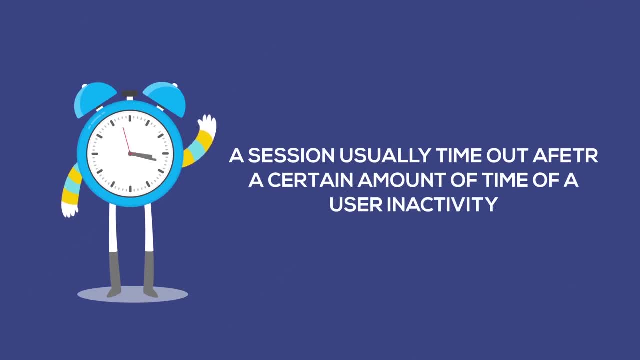 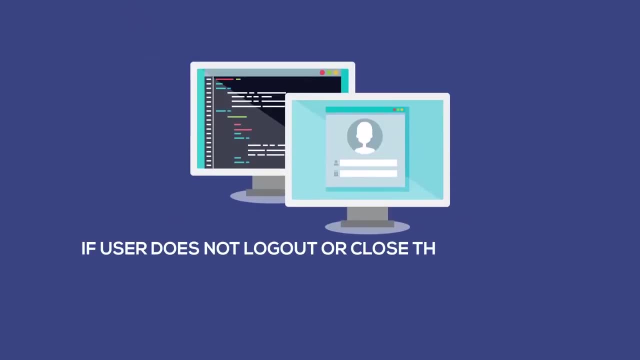 of time of a user inactivity. So it's best practice, security practice, that application knows that the timeout a session, because if a user does not log out or close their browser, by the way, closing their browser automatically kills the session. And if they don't do either, 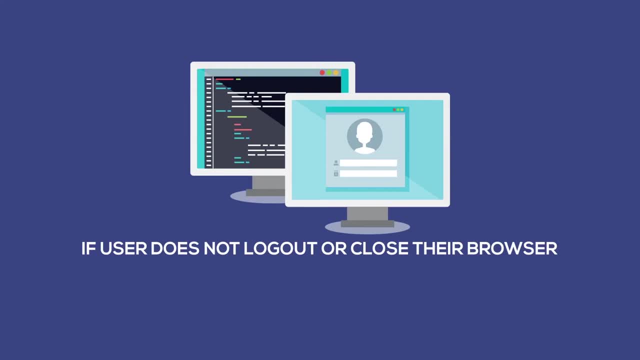 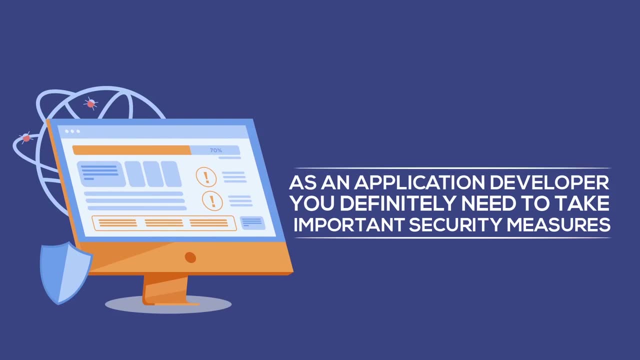 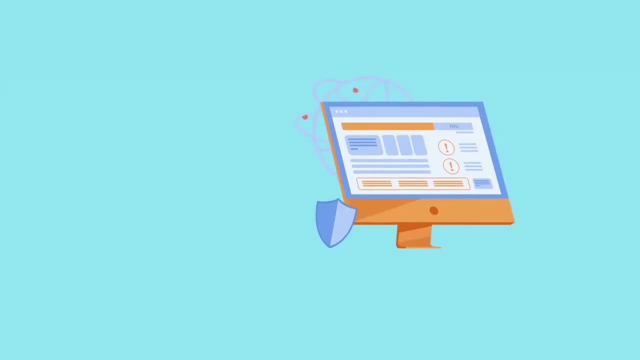 of that. you want to timeout that session before has a high chance of being hijacked And in the real world you got to take as an application developer. you definitely need to take important security measures to make sure session hijacking is mitigated. The last thing you want is a 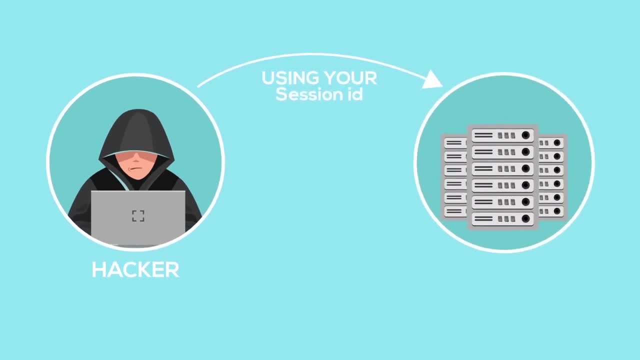 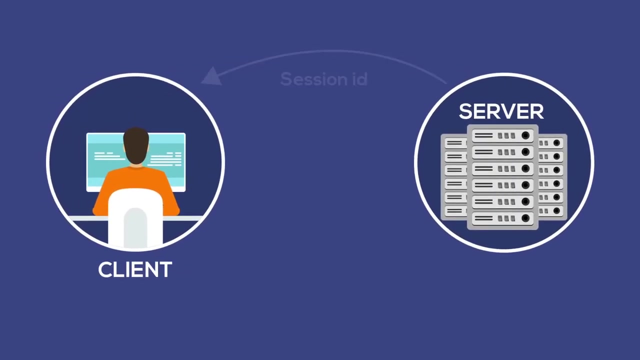 hacker getting control of your session ID and making requests on your behalf, because then it can get your get, get your data right. So that's bad. You don't want that to happen. So, like I said, session: the server sends the session ID to the client. the client sends the session ID back to. 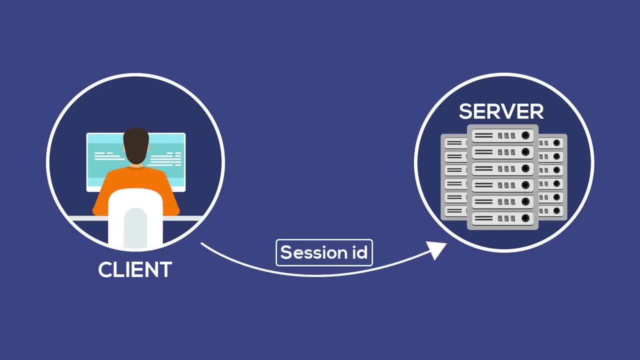 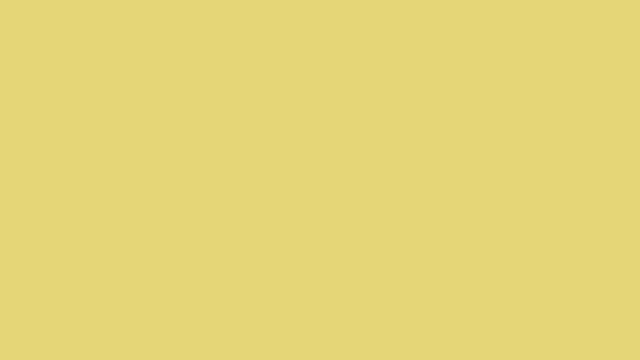 the server And the server uses that session ID to get the data in that data store. So that session ID is very important And think of some use cases like shopping carts, the store 10, buried data. you can store that in the server. Also use authentication. So instead of having a